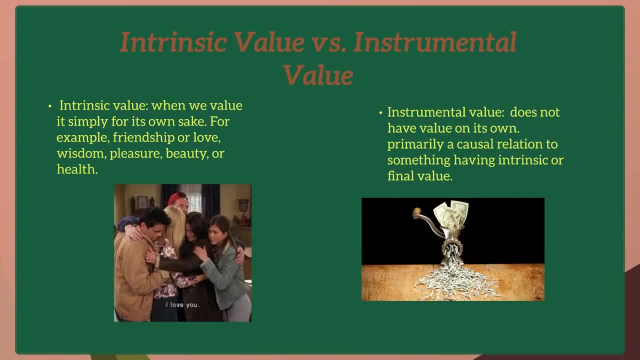 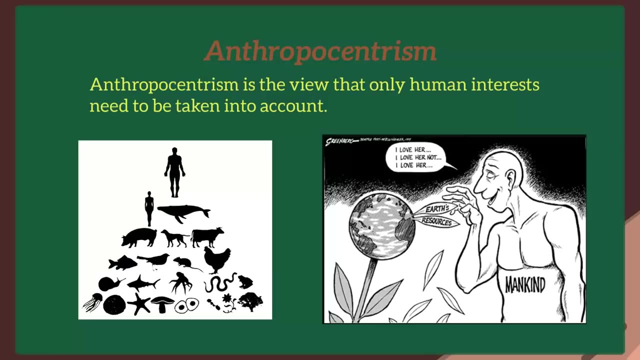 paper, but when you add instrumental value to it, it becomes a major social and economic tool. The three main types of ethics we see today are anthropocentrism, biocentrism and ecocentrism. Anthropocentrism is the view that only human interest needs to be taken into account. 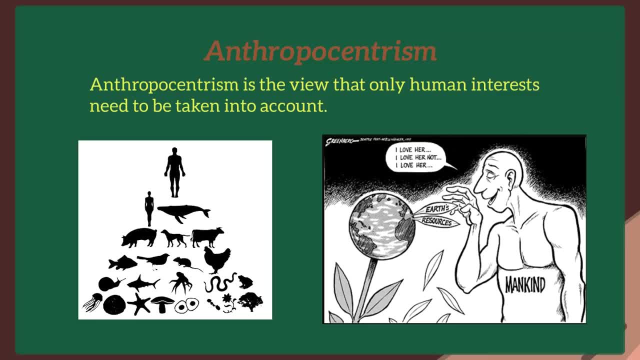 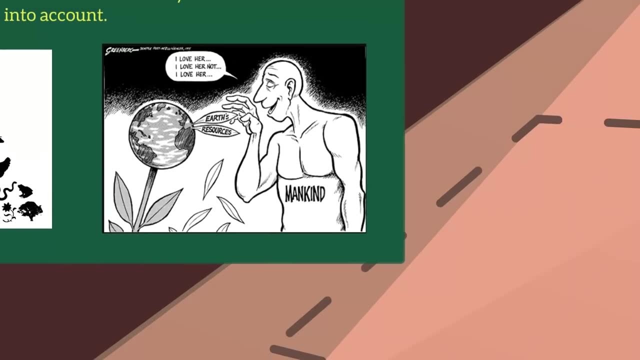 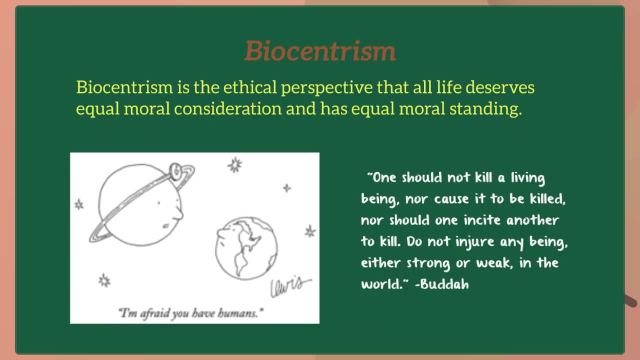 Many traditional Western ethical perspectives are anthropocentric and assign a significantly greater amount of intrinsic value to human beings than any non-human beings. They justify the protection of human interests and well-being at the expense of non-human things. Biocentrism is the ethical perspective that all living organisms should be considered. 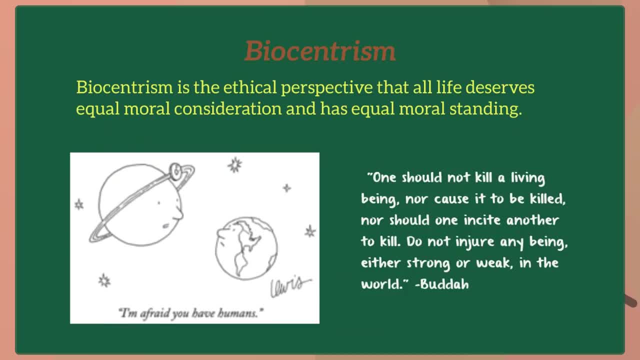 as equals. Critics highlight that strictly biocentric ethics will conflict with a more ecologically influenced environment. Protecting individual lives is the most important aspect of biocentrism. Biocentrism may lead to harm rather than protecting the integrity of ecosystems. 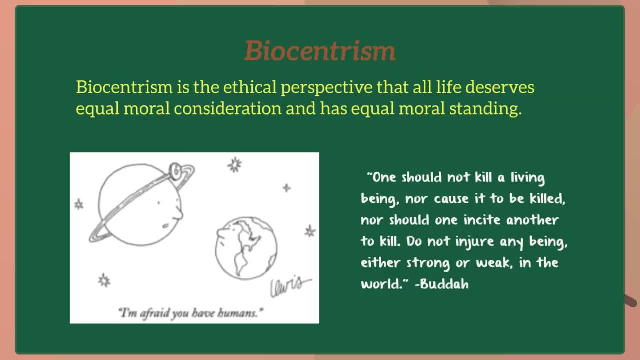 The evidence given by critics is that there is a need to remove invasive species for ecosystem health. It is, of course, always open for the biocentric approach to accept the conflict by simply denying the value of ecological wholes and shifting the focus of biocentrism to have 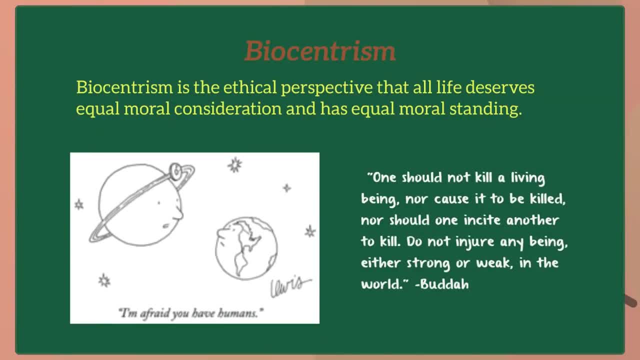 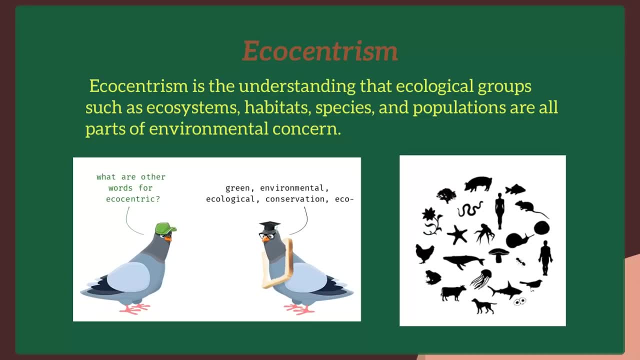 only incidentally overlapping concerns with environmental ethics. The last environmental ethic is ecocentrism. Eccocentrism is the understanding that ecological groups such as ecosystems, habitats, species and populations are all part of an environmental concern. This approach determines that preserving the integrity of the ecosystems and the survival 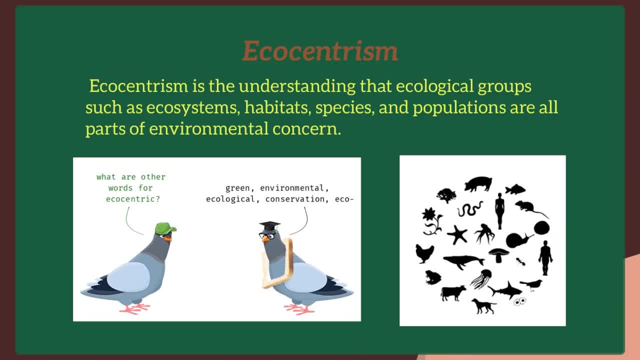 of species and populations is environmentally more crucial than protecting the lives of individual elements of an ecosystem, ecosystem or members of a species. Ecocentric environmental ethics often would overlook destroying the lives of individuals as a legitimate means of preserving ecology as a whole. so, members of an overpopulated 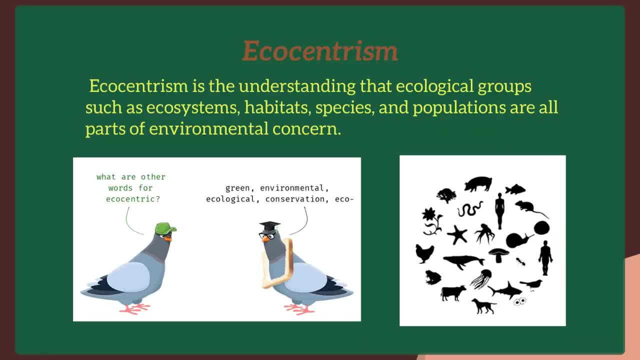 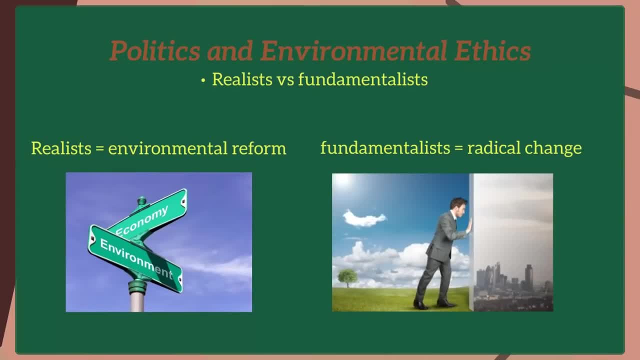 herd or killing an invasive non-native plant or animal species can be justified. There has always been a large debate discussing what is legal and ethical in regard to politics and the environment, The emergence of philosophies to underpin animal rights activism and the puzzles over 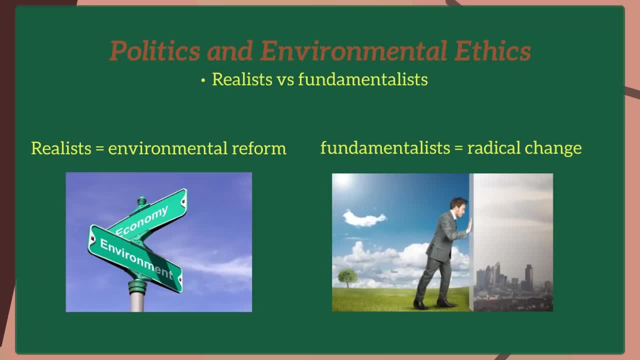 whether an environmental ethic would be something new rather than a modification or extension of existing ethical theories were reflected in wider social and political movements. The rise of environmental or green parties in Europe in the 1980s was accompanied by almost immediate clash between groups known as the Realists versus Fundamentalists. 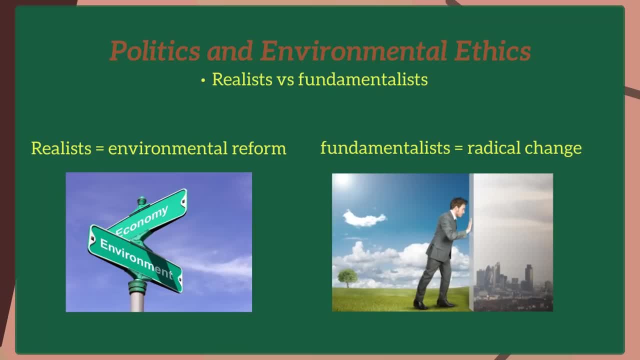 The Realists stood for reform, environmentalism, working with businesses and government to soften the impact of pollution and resource depletion, especially on fragile ecosystems or endangered species. The Fundamentalists argued for radical change, the setting of stringent new priorities and even the overthrow of capitalism and liberalism. 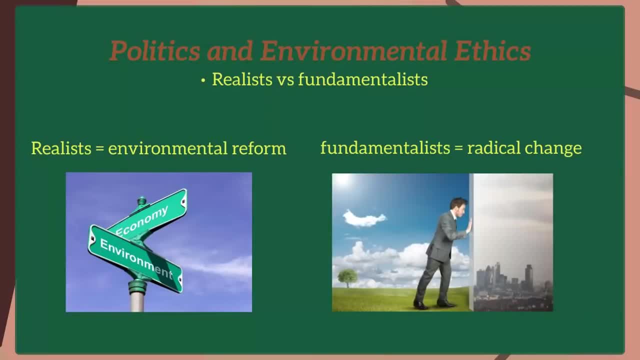 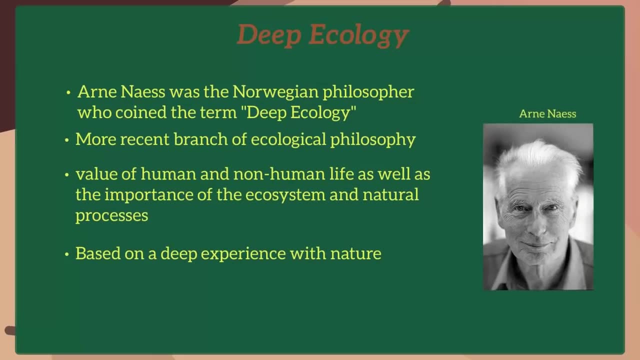 liberal individualism, which were taken as the major ideological causes of anthropogenic environmental devastation. Deep ecology is a somewhat recent branch of ecological philosophy that considers humankind as an integral part of its environment. The philosophy emphasizes the interdependent value of human and non-human life as well. 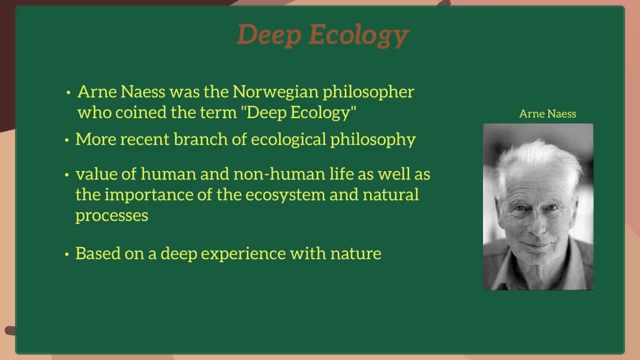 as the importance of the ecosystem and natural processes it provides. It provides a foundation for the environmental and green movements and has led to a new system of environmental ethics. In the 1960s, having read Rachel Carson's book Silent Spring, Arne Aeneas was moved. 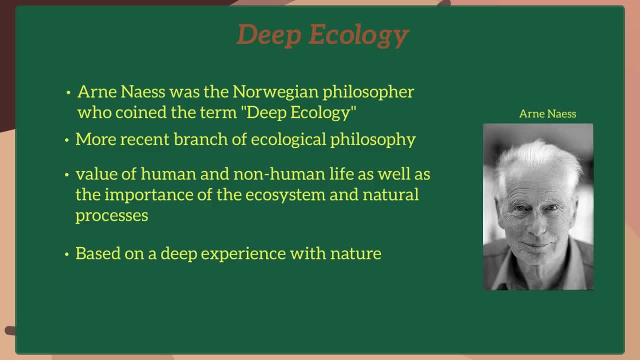 to apply his formidable philosophical skills to understanding the ecological crisis and its resolution. Since becoming the youngest ever person in the United States, Arne Aeneas has been studying the ecological crisis and its resolution Since becoming the youngest ever professor of philosophy at the University of Oslo. while still in his 20s, Arne Aeneas has 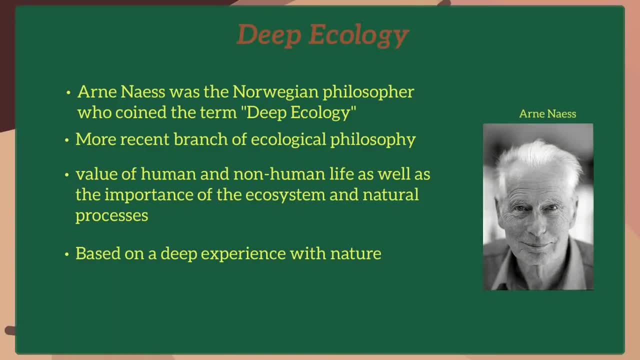 revealed his brilliance by studying and writing extensively in many fields, including semantics, philosophy of science and the works of Spinoza and Gandhi. His approach to ecology bears the stamp of his life's experience as a philosopher and the truest sense, and it shows in his role in the development of deep ecology and the 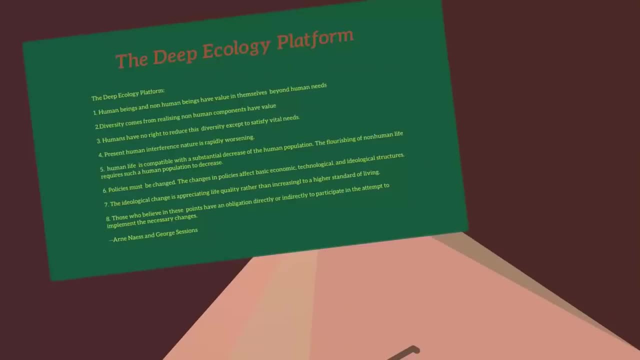 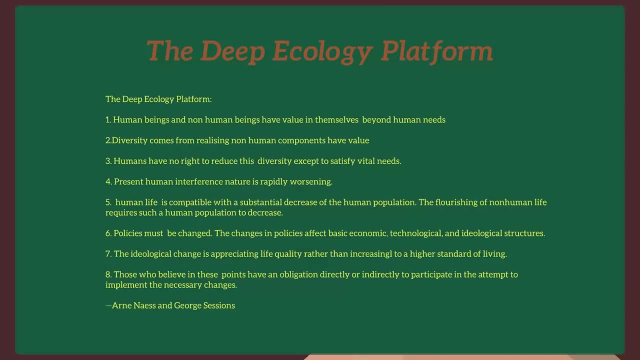 coining of the phrase The Deep Ecology Platform. Naas and George Sessions both developed eight guidelines to practicing deep ecology and they are called the Deep Ecology Platform. The well-being and flourishing of human and non-human life on Earth have value in themselves. These values are independent of the usefulness of the non-human world for human purposes. 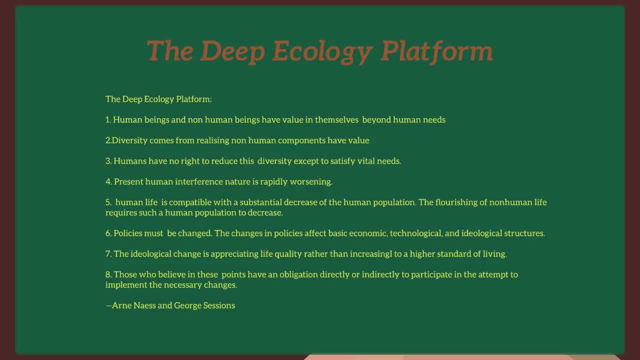 Richness and diversity of life forms contribute to the realization of these values and are also values in themselves. Humans have no right to reduce this richness and diversity, except to satisfy vital needs. Present human interference with the non-human world is excessive and the situation is rapidly. 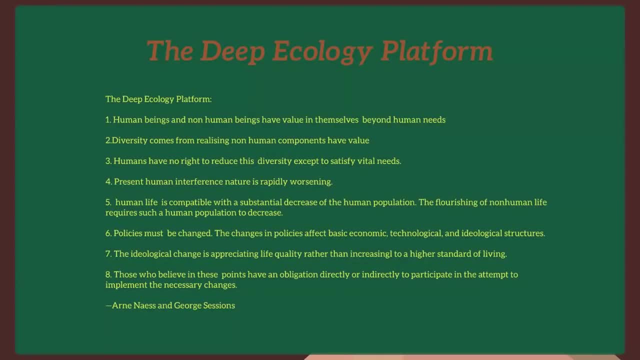 worsening. The flourishing of human life and culture is compatible with the substantial decrease of the human population. The flourishing of non-human life requires such a decrease. Policies must therefore be changed. The changes in policies affect basic economic, technologic and ideological structures. 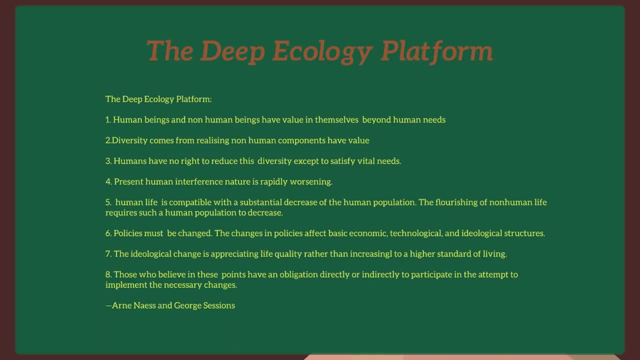 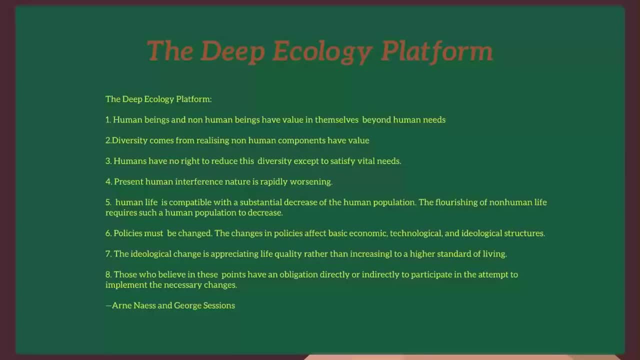 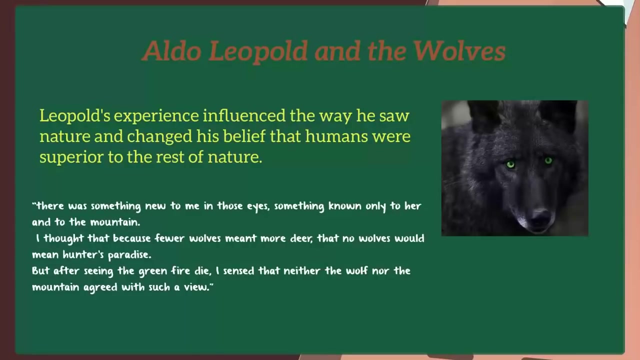 ortion of economic diversity, The aquellos who enjoy clapping dixion, iniquity, dixation, iniquity King and Euphoric Proverbs. 2mus often what gets a person started along a deep ecological path. Another founder of deep ecology. 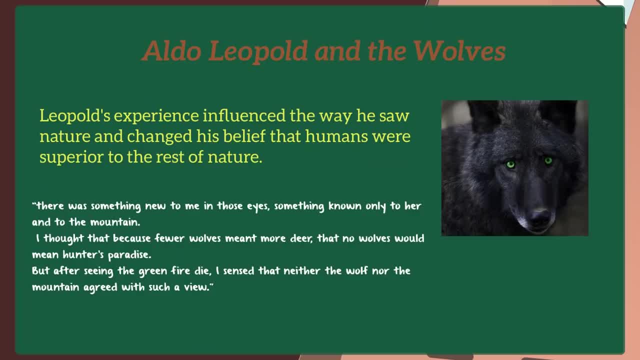 is Aldo Leopold. In his book A Sand County Almanac, he provides a striking example of how experience can bring forth important, life-changing realizations. For Leopold, the experience was of a sufficiently intensity to trigger a total reorientation in his life's work as a wildlife. 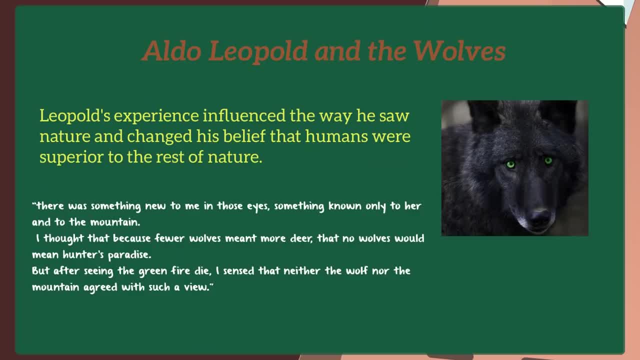 manager and ecologist In the 1920s. he had been appointed by the US government to develop a rational scientific policy for eradicating the wolf from the entire United States. The justification for this intervention was that wolves compete with sport hunters for deer, so that fewer wolves 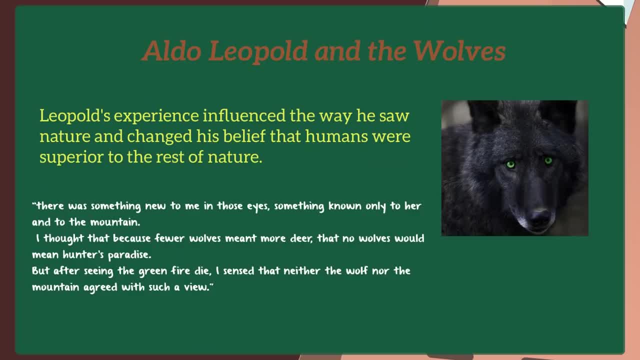 would mean more deer for hunters. As a wildlife manager of those times, Leopold still held to the unquestionable responsibility of being a wildlife manager and ecologist. In his book A Sand County Almanac, he것도 a pre-стаught-up supercomputer and investigator who was to assign the task to 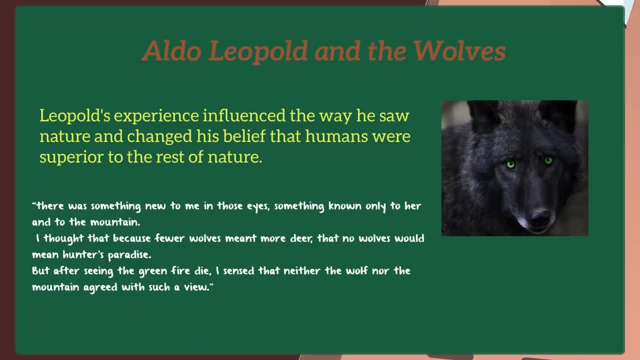 a skilled hobbyist that was often paying bonds of the directly틀 in the bird's- tellement. When Leopold arrived, he had a questioning belief that humans were superior to the rest of nature and were thus morally justified in manipulating it as much as was required to maximize human 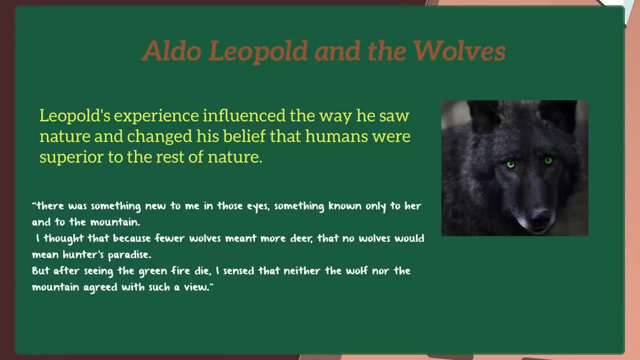 welfare. One morning Leopold was out with some friends on a walk in the mountains. Being hunters appeared to be some deer fording at the torrent, but they soon realized that it was a pack of wolves. they took up their rifles and began to shoot excitedly into the pack, but with little accuracy. 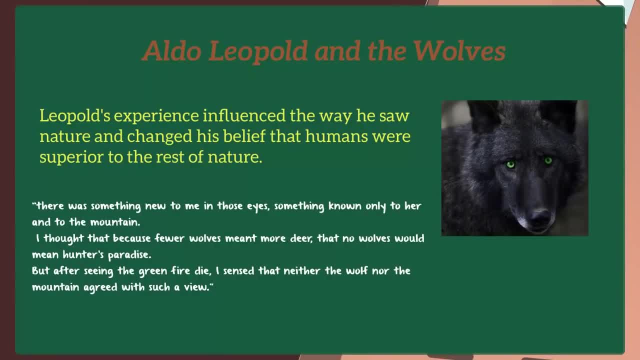 eventually, an old wolf was down by the side of the river and real leopold rushed down to glow at her death. what met him was a fierce green fire dying in the wolf's eyes. he writes in a chapter entitled thinking like a mountain that there was something new to me in those eyes. 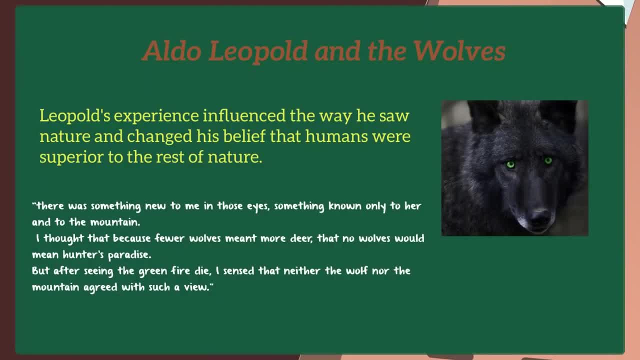 something known only to her and to the mountain. i thought, because fewer wolves meant more deer, that no wolves would meet hunter's paradise. but after seeing the green fire die, i sensed that neither the wolf nor the mountain agreed with such abuse. this compelling story really paints a picture of how leopold was influenced by this experience and